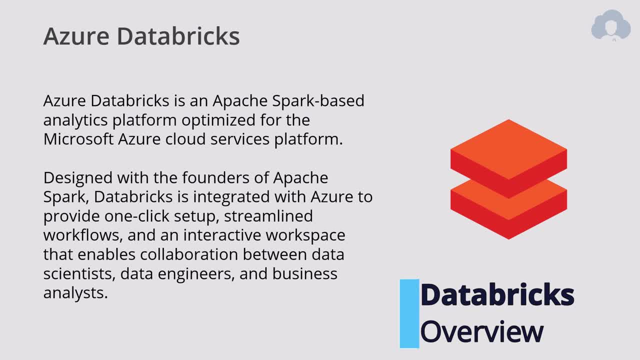 So Azure Databricks. What is Databricks? I think the easiest to explain Databricks is: it's the big data technology that Microsoft brought as one of the services in Azure. It's a very cool platform that is based on Apache Spark. Why is it cool? Because it is created and designed. 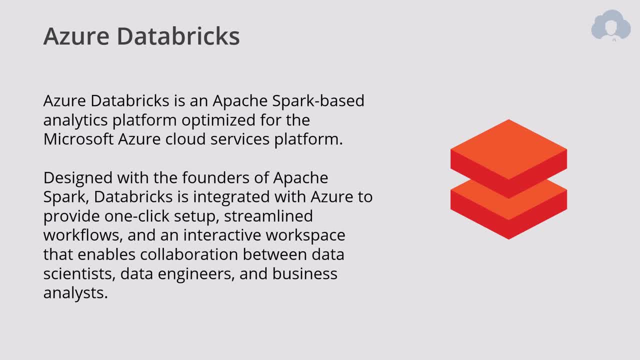 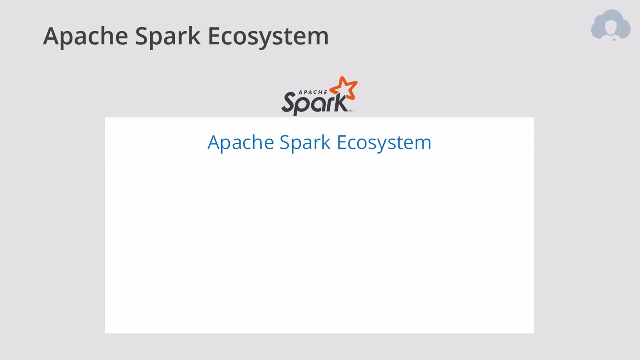 by the same people who actually created Apache Spark And since Apache Spark is one of the leaders of big data technologies on the market, it really promises fast transformations in the cloud. So, since it's based on Apache Spark, the key features that you will see in this video are the following: 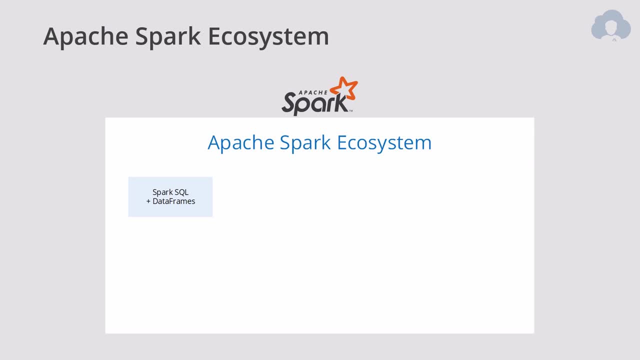 So what you would get from this are, first of all, Spark, SQL and DataFrames. This is a library that allows you to work on your structured data as pretty much tables in any system that you've been working on already. Additionally, you have some services that allow you for streaming of the data. 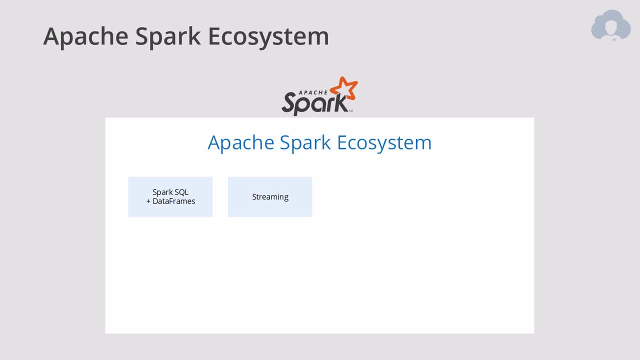 So if you're doing IoT or live event applications, this is one of the great examples of how you can perform transformations on the live system. You also have machine learning library which allows you to do machine learning type of transformations, prepping and training models using Spark itself. 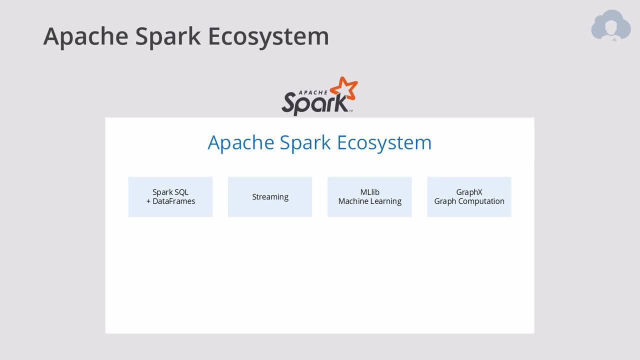 You also have GraphX, So if you're doing some social media type of applications, then this is also a great place to do so, And everything is basing on Spark core API, which means you can use R, you can use Spark SQL, which is a little bit different than normal SQL. 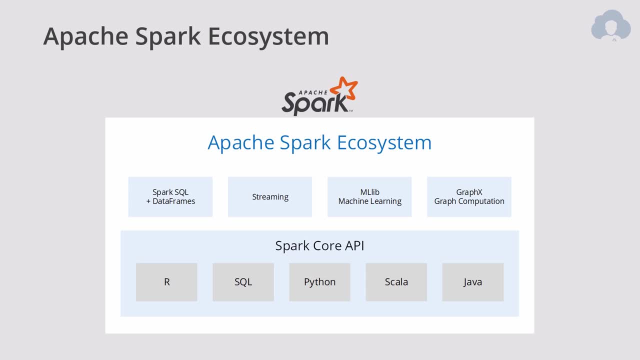 It's more limited, but it's still very powerful. So if you know SQL, that could be a very good feature for you to use without needing to learn any other different language. You also have Python, Scala. Those are the two main languages that you will be using when 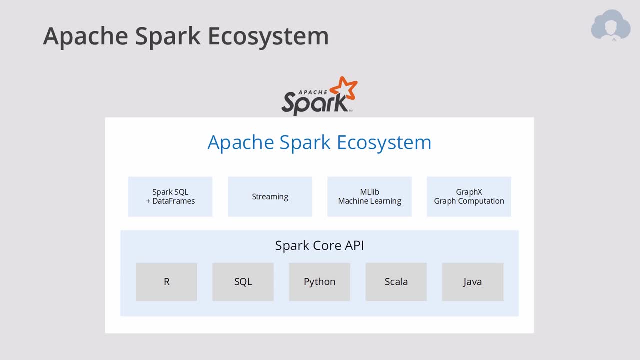 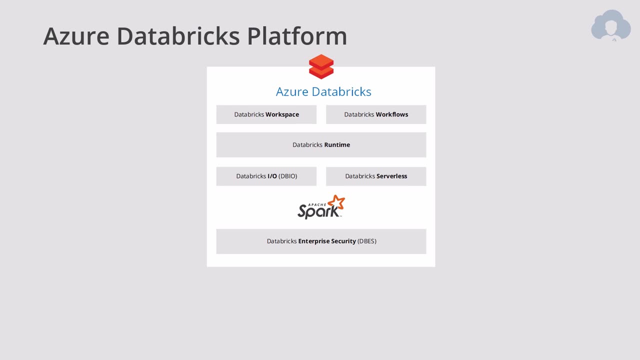 developing in Databricks, but you also have Java if you need to do that. Databricks as a platform has a lot of features itself. Besides being Apache Spark based, it also has a runtime. Runtime combines those features together into a singular platform which delivers you workspaces and places where you 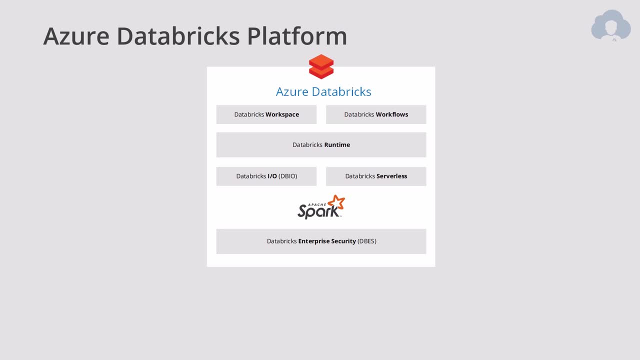 can collaborate with your friends and colleagues on your scripts. If you have multiple scripts, you can combine them into workflows. Workflows can be nesting of the scripts, scripts calling another scripts- basically a simple ETL, And also you have a DBIO. 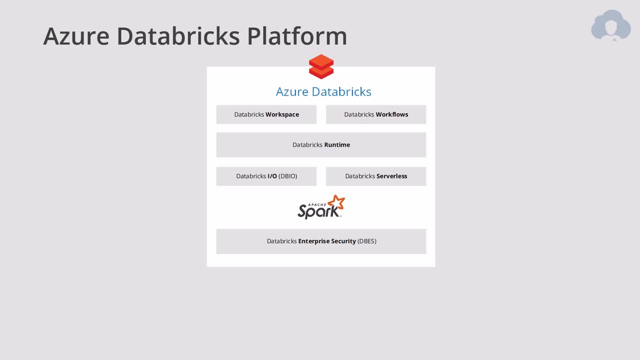 which is Databricks input output library allowing you to easily connect to multiple services, both in Azure and not only, like Apache, Kafka and Apache- sorry and Hadoop- But also Databricks- has something called Databricks serverless. What this really means is that 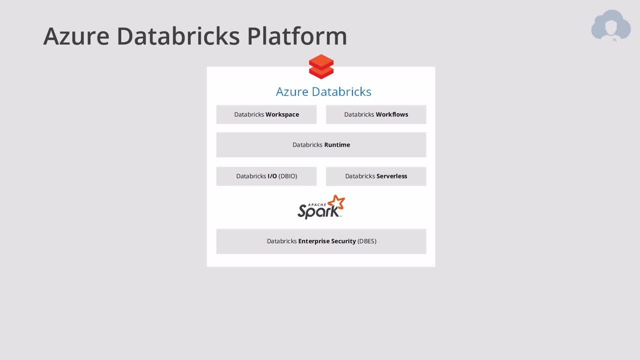 when you work with Databricks, you just specify: what kind of server do you want, how powerful it is, how many of those servers do you want, what is the runtime that you want on it, And that's it. Databricks as a platform will manage handling. 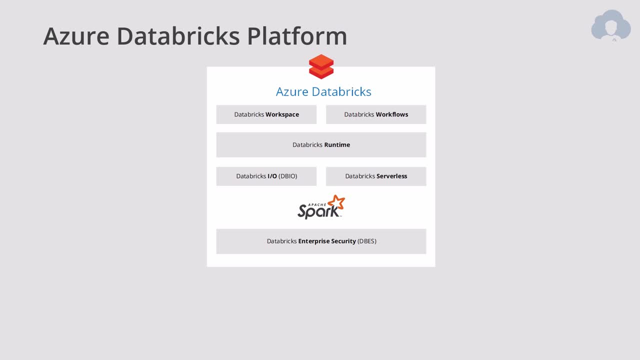 and creation of that clusters for you without you needing to manage them at all. And lastly, there's something called enterprise security. So Databricks is integrated very well with Azure and Azure Active Directory. So handling all those accesses, credentials, authorization- everything is basing on Azure. 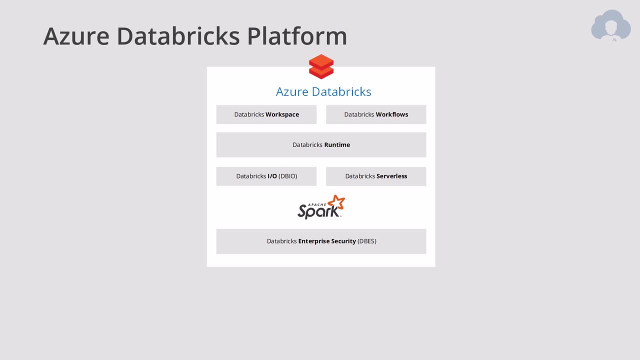 IT So you can just use your corporate credentials and identity to use Databricks itself. There are a lot of storage solutions that they can connect to, but the five main ones that has native connectivity is a blob storage, data lake, data lake in both version one and two, SQL data warehouse, Apache, Kafka and Hadoop. 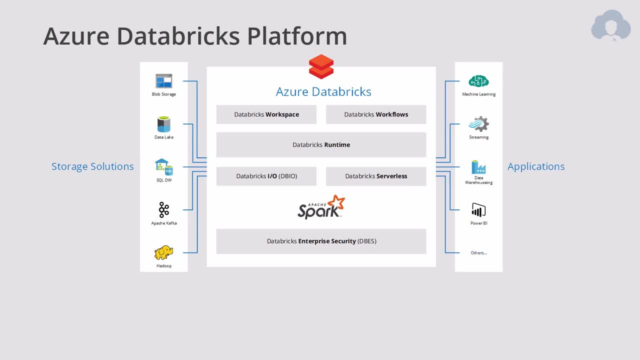 We already mentioned some of those, But also there are several applications that you can use Databricks for. The most common ones are machine learning scenarios, streaming scenarios, data warehousing- so your typical ETLs- prepping the data- and Power BI, which is very common. 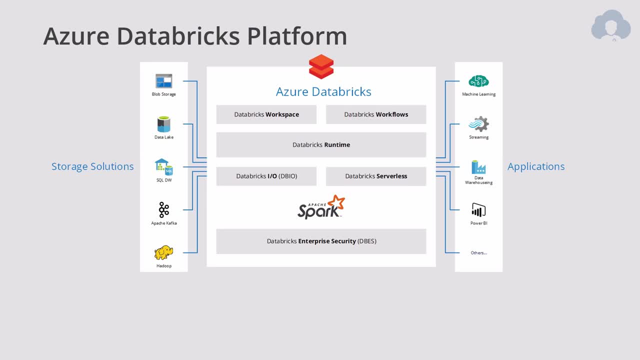 This is a common case recently, But there are many, many other applications that you can use Databricks for. Since this is a collaborative platform, it is really easy for users to use it. There's a UI that they can use. It's very- I would say it's very- simple. It's very simple. 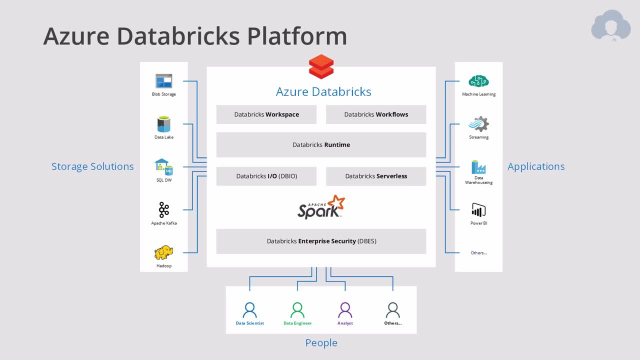 once you know the platform. But since there is a UI, you don't really have to be technical savvy in order to use it. So your typical data scientists, engineers, analysts- once they learn the platform, it's very easy for them to use Databricks as well. 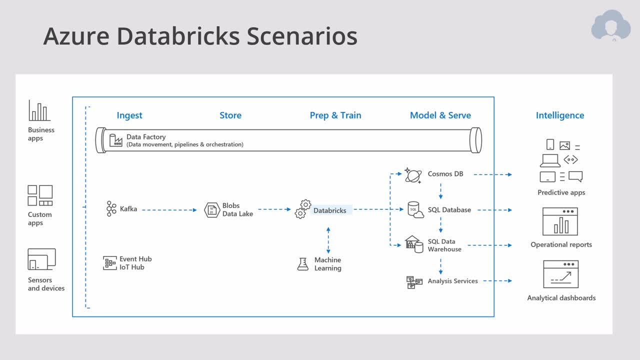 The typical scenario that you would see Databricks in is during the prepper train for machine learning or your typical prep, which is part of the ETL. You normally have ingestion layer, so either Data Factory, Kafka, IoT Hub, Event Hub, something. 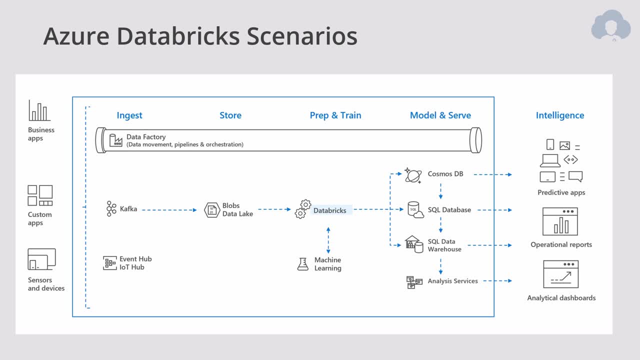 gathering your data from external systems and putting it either on a blob or data lake. So this is where the Databricks come in. Usually, Databricks will grab that data from the blob or data lake, transform it or train the models, if it's machine learning scenario, and put it in some 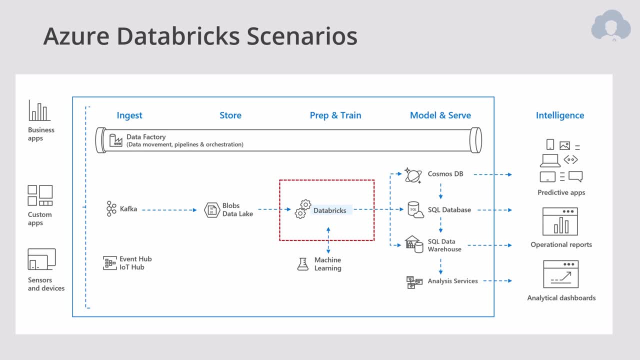 sort of database. It can be their SQL database, Cosmos DB, data warehouse, or maybe even analysis services. Or you, of course, can put it back on a blob storage if you want to. That's up to you. Since this is a scripting platform, you can actually design this logic as you fit to. 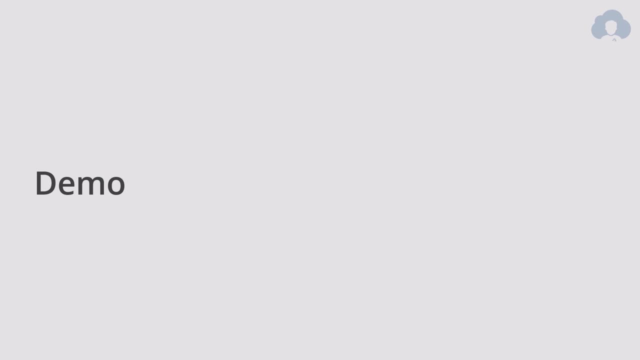 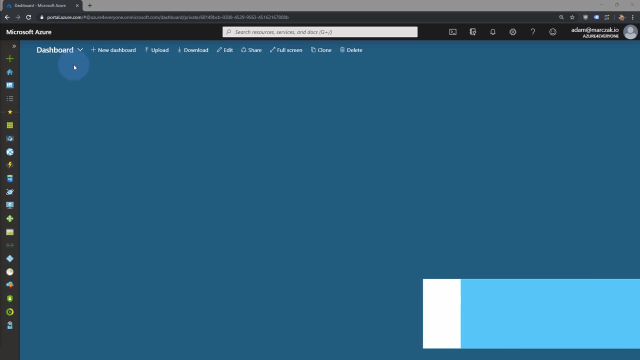 So, without further ado, let's go into the portal and start doing some demos. So in Azure, we will need a couple of things. First of all, we're going to need to create the Databricks. In order to create Databricks, hit on Create Resource and type Databricks. 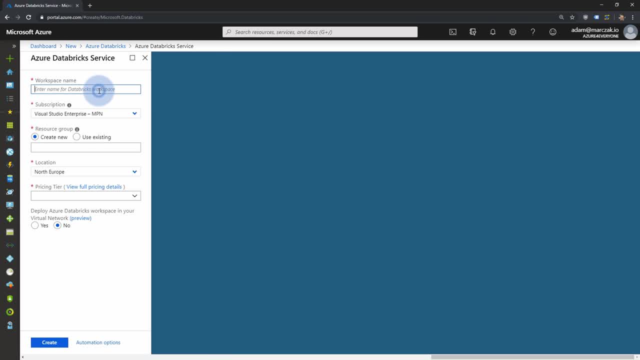 And hit Create. when you find the template And just give it a name- I'm going to call it A4EDB- Intro- And then click on Create. And now we're going to create a new database And we're going to need to provide a resource group. This is where your Databricks workspace. 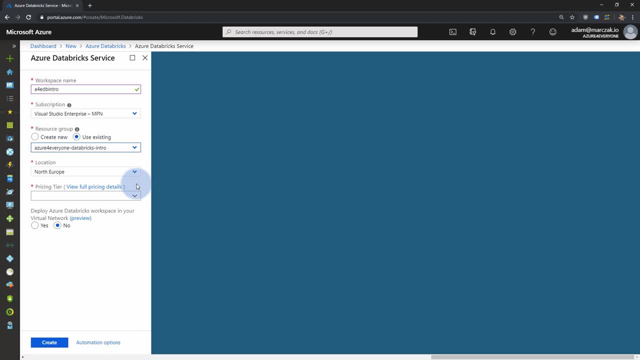 will be residing, So I'm going to pick my resource group that I created previously. I'm going to leave location of Europe. This is the closest data center to me. In the pricing tier, I'm going to select Trial. Please note that this is the trial. 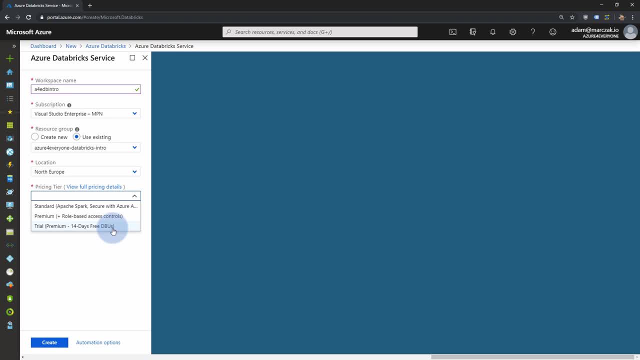 The 14 days free DBU that you're getting is only the licensing cost for the Databricks that you're not going to pay for, But you're still going to pay for the virtual machines itself You can deploy to virtual network as no, because this is not the part of the training for today. 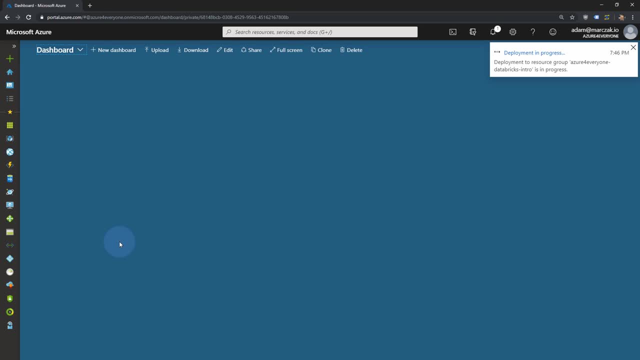 So I'm going to hit Create And the second resource that we're going to need today, because we're going to be transforming data And, as we've seen during our presentation, we need to ingest it from somewhere. I'm going to grab a blob storage for that. 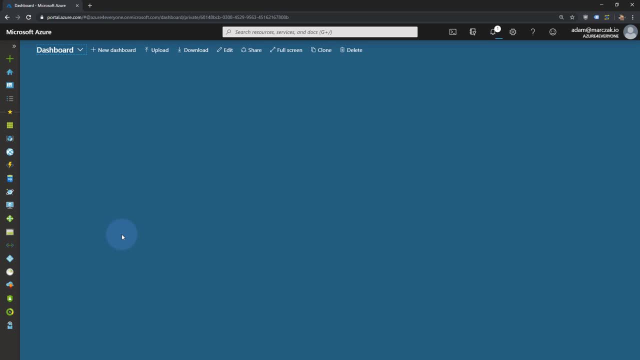 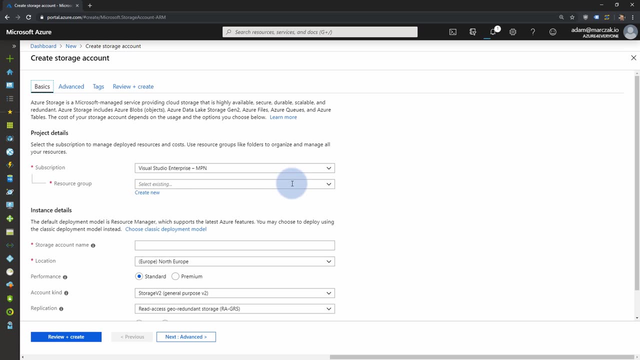 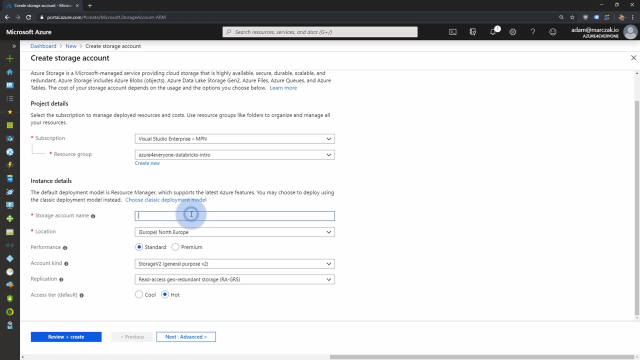 where I'm going to be uploading files for our processing purposes. So I'm going to hit plus and find the storage account. It's quickly here. I'm going to provide a name, but first I need to select the resource group. So the same resource group as previously. I'm going to also leave North Europe. 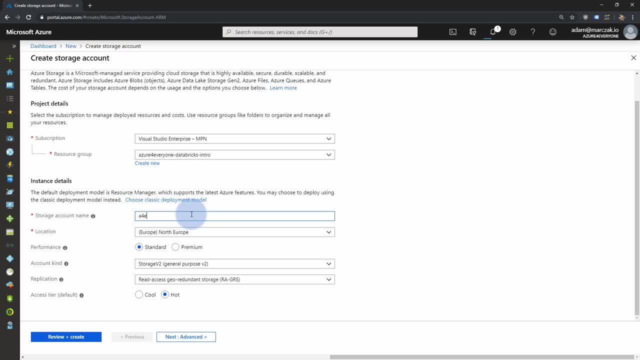 and I'm going to provide A4E DB intro name And everything else is going to be left as default. Of course, you can change replication if this is just the ingestion layer, So you're going to get better performance. So, if I'm going 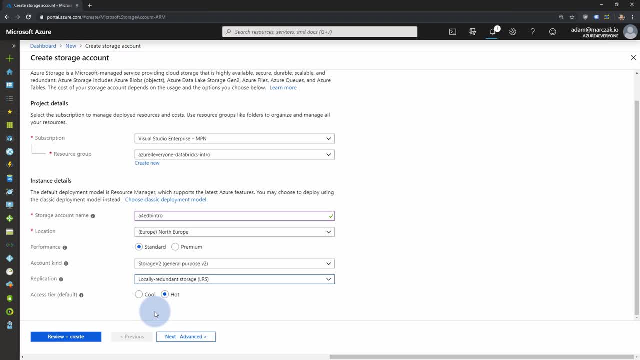 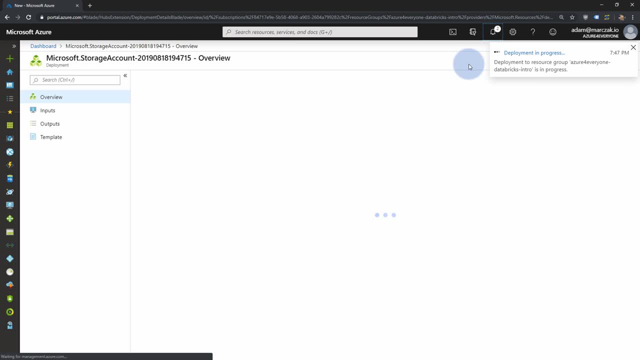 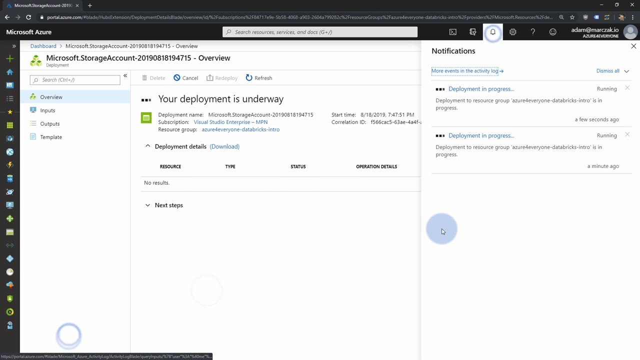 to leave locally redundant storage. this is the cheapest and the fastest storage that we can get, So let's hit review and create and hit create. Provisioning of resources takes about a minute or two, So I'm going to speed this up. So the provisioning finished so we can go to our Databricks resource. 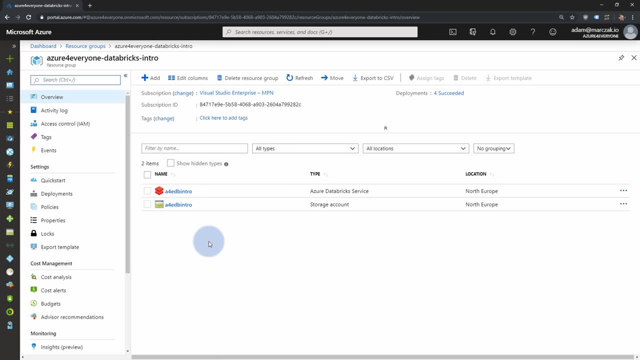 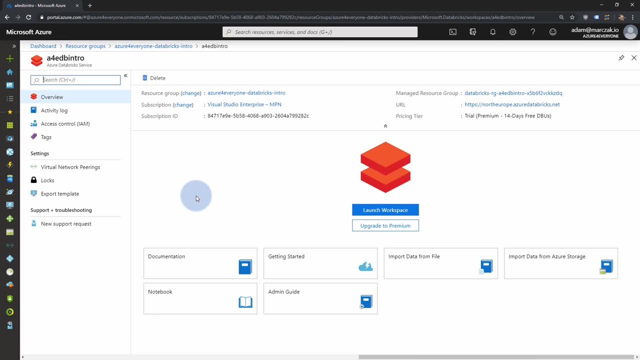 So let's go to resource group: open our resource group, And those are the two resources that we just created. So I'm going to hit on the Databricks resource And I'm going to hit on launch workspace. This is going to bring me to the separate portal. 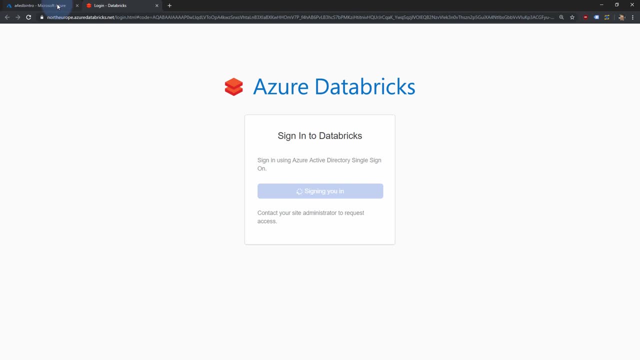 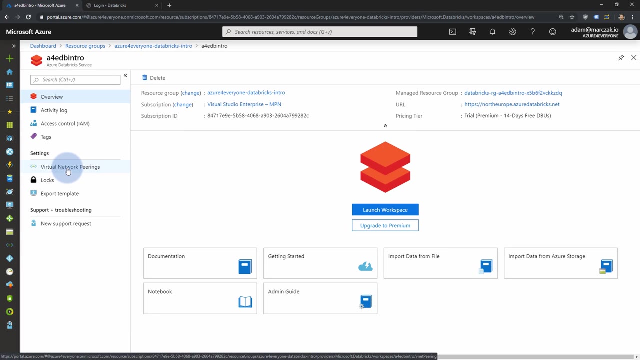 the portal where you're actually going to be doing all the work. There's actually literally almost nothing that you can do related to Databricks here in the Azure portal itself, other than some virtual network connectivity. So let's go back to the Databricks platform. 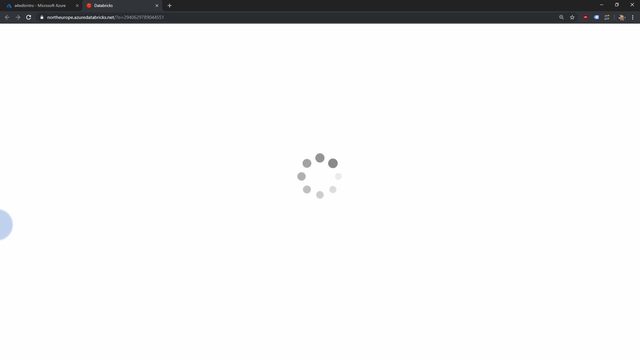 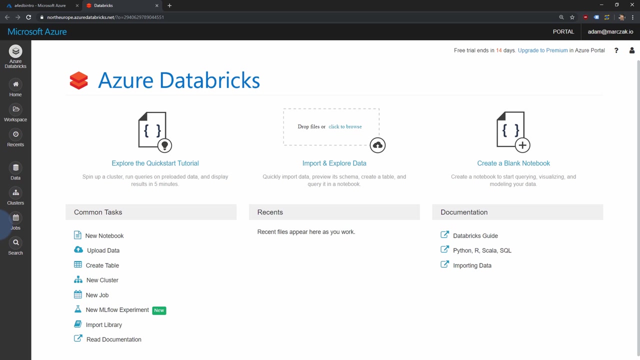 This initialization takes about a minute or two as well, but I've seen the rare scenarios where this sometimes takes up to an hour. So if this happens for you, just patiently wait or maybe come back later. So in the Azure Databricks portal, you can do here a couple of things, but the most important 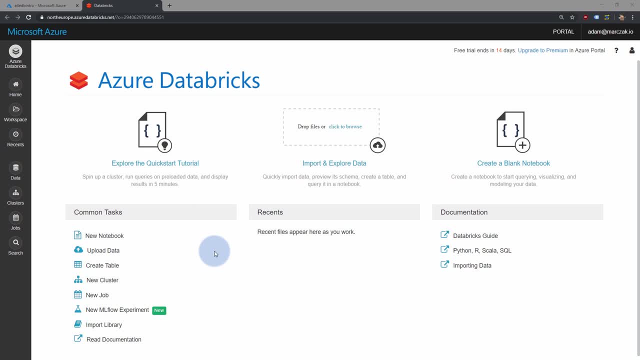 that we're going to be doing today is running the scripts and creating clusters. Clusters are the workloads that you're going to be running on the servers that will be executing your scripts. So what we need to do right now is create new cluster. 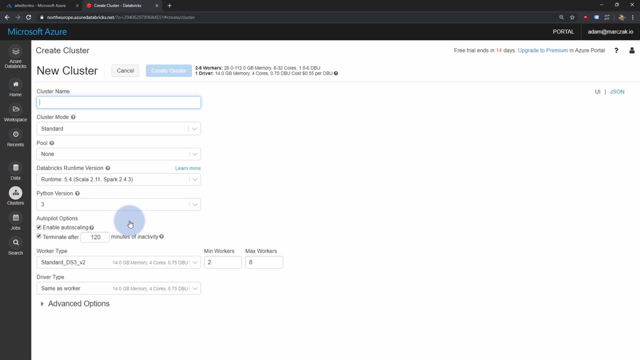 You can quickly hit here new cluster and provide details of your cluster. I'm going to call it demo because the name is just important for me right now, But in case you're collaborating, always pick meaningful name. What is the cluster mode? Standard or high concurrency? 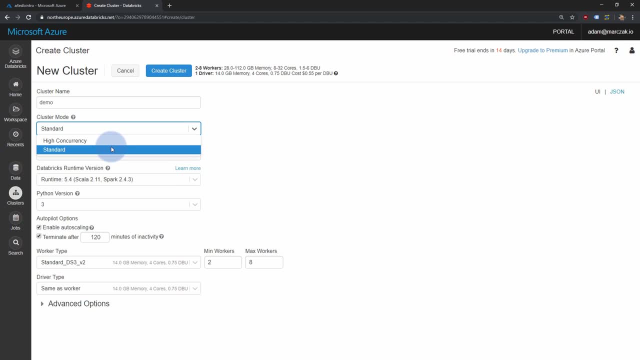 If multiple users are working on the same cluster, it is advised to use high concurrency. If this is a cluster for your ETO transformation, just pick standard. Next you have pool. I'm going to leave this as none, And we have database runtime version. 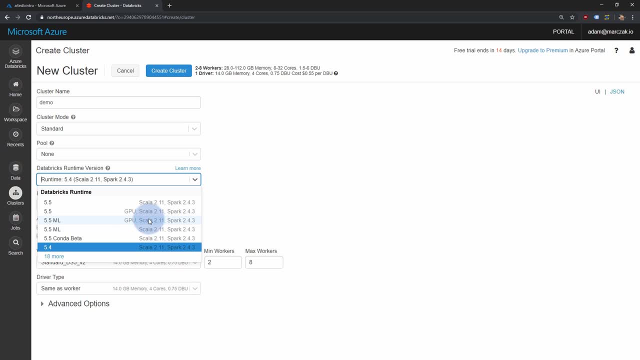 For the demo purposes, leave this as default. But, as you see, you have a lot of Databricks runtimes, So if you need Scala or Spark in a different version, you can always find it here. So I'm going to leave runtime 5.4.. I'm going to leave Python version as 3.. 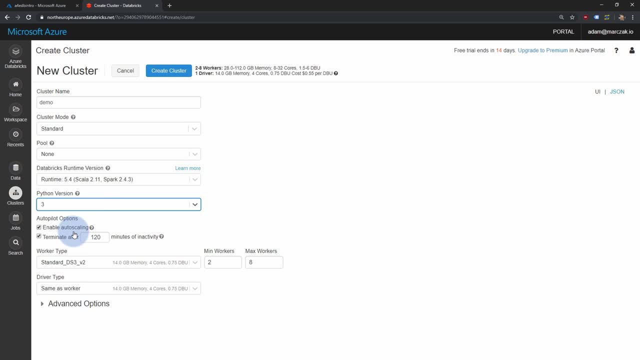 And the next two options are very important. First of all, you have enable autoscaling. So if you're running workloads that sometimes needs more and less power, you can enable autoscaling And this will pretty much bring from 2 to 8 servers for your processing needs. 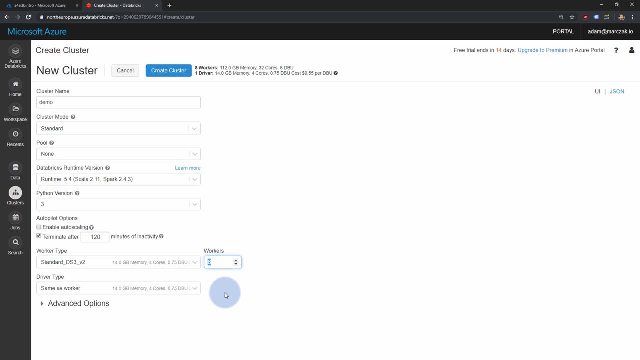 In our case, I'm going to disable this and change workers to 1.. The reason for doing that is because our scripts are very, very small And if you're going to pick more servers, not only you're going to pay more, but the execution will take more time, because the time it will take to split the task 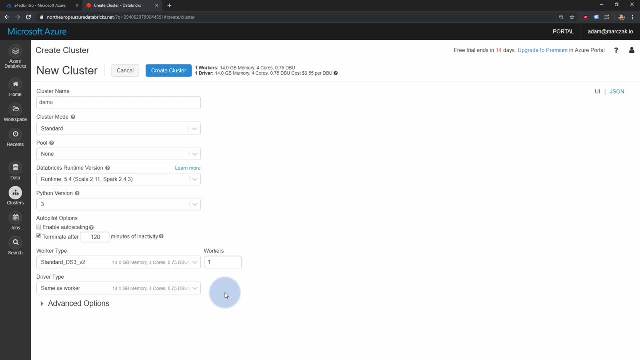 into two servers and combine the results together is larger than the actual work that needs to be done. So I would advise, always for training purposes, to just grab non-autoscaling cluster with only one worker, And there's very good feature here called terminate after. 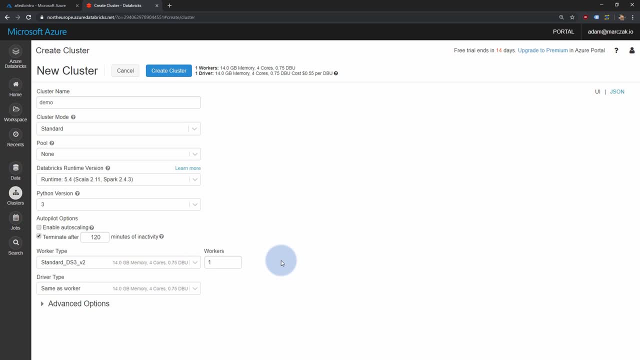 That means if you have a cluster and you're finished processing workloads and you went home, you stopped processing, it will automatically delete the cluster for you. You don't pay anything at all, And this is why, even though you pay additional license for the 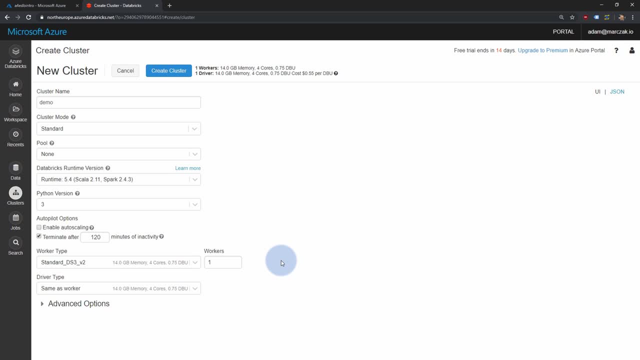 Databricks itself, you usually end up paying less than for the usual services that transform the data, So I'm going to leave this to 30 minutes. So if for 30 minutes I'm not using this, it's going to delete it And I'm going to pick the smallest server available. 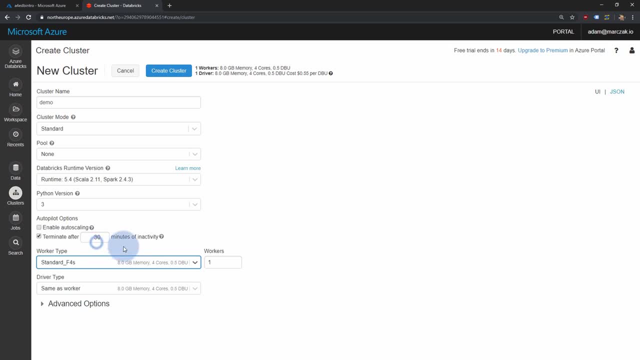 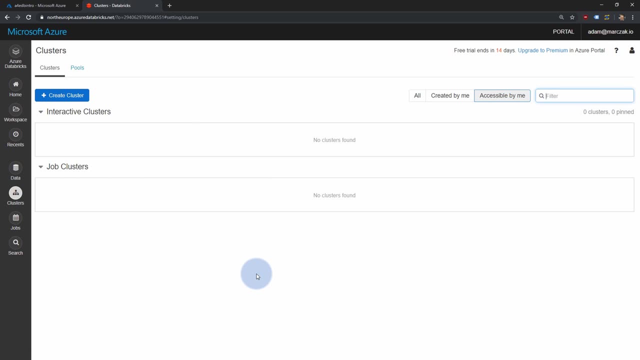 And I think this is the F-series. F4S is the smallest server, So I'm going to pick the smallest server that you can use and hit Create Cluster. After doing so, your server will be up, probably between one and five minutes. 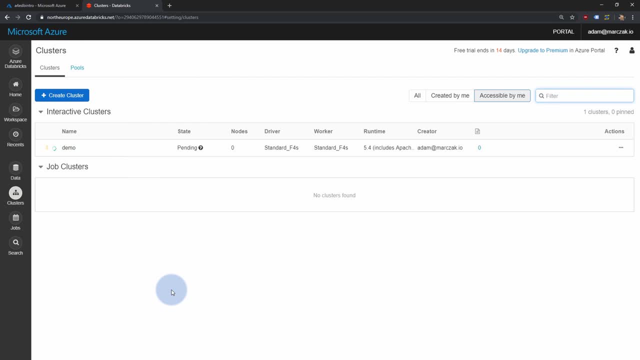 So again, I'm going to speed this up. So, since our cluster was created and it's running notice, first of all, you have two nodes. Two nodes are because there's always master and a worker. Worker is the server, A virtual machine that runs all the scripts that you create. 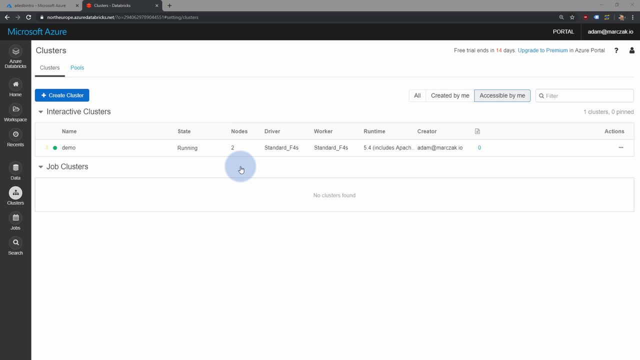 And the master is virtual machine that orchestrates all the scripts execution and splits them across multiple workers, if you have more than one. So let's go to workspace and start creating our scripts. So hit on the workspace. go to users. hit on your username. 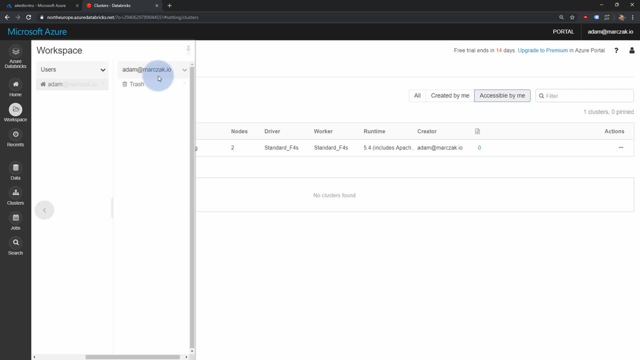 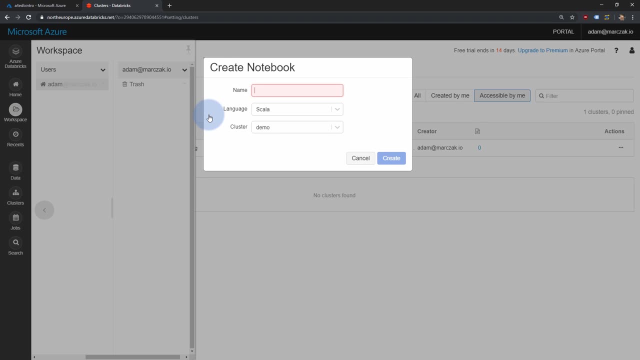 And this is where I'm going to be doing my work right now. This is my personal workspace where I can create notebooks, So I'm going to right-click, hit Create Notebook, And notebook is basically your scripting language. So I'm going to pick Python and I'm going to type Demo1.. 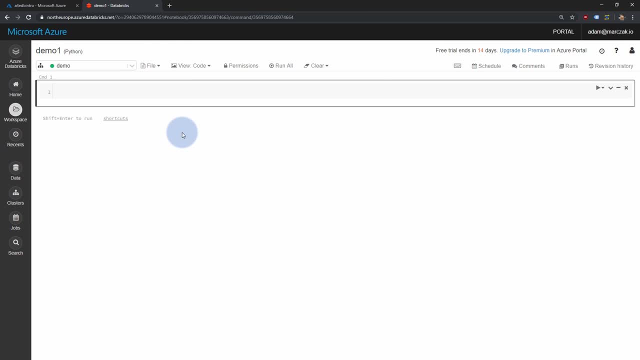 This is going to be name of my notebook where I'm going to be writing my scripts, And, of course, this is not the demo of how to write Python and Scala scripting. Therefore, I prepared all the scripts beforehand, So the first demo in Python that we're going to run is prepared by Microsoft. 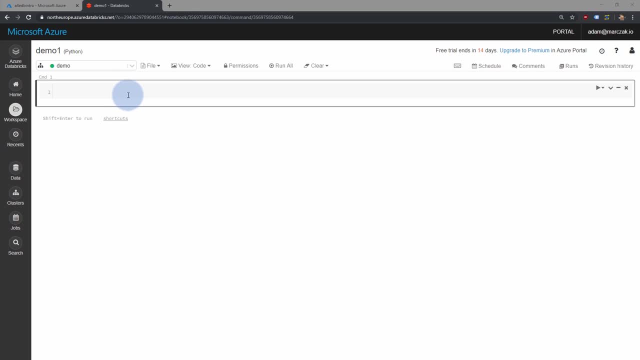 Microsoft gave the data that you can run via Python, So I'm going to run it very quickly to see how Databricks works. So I'm just going to copy-paste that. So first of all, I'm going to create four variables. 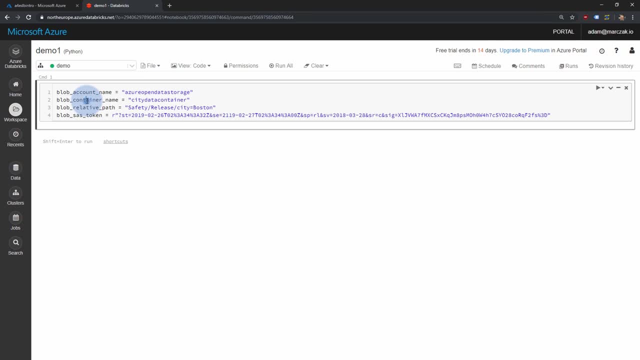 So we're going to create the blob account called Azure Open Data Storage to the container relative path and provide SAS token. SAS token is your key that we're going to use to authorize to this container and pull this Boston data In order to run this block. 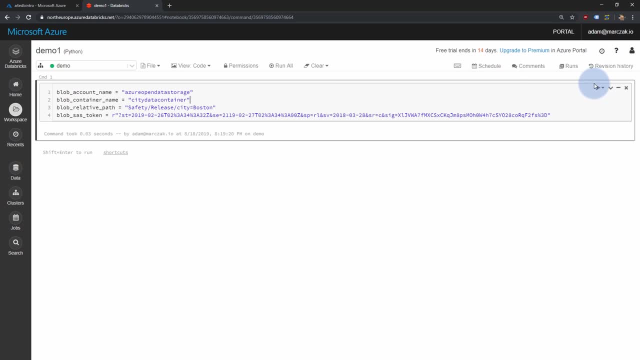 you simply need to hit control enter, or you need to hit this run cell button here and hit run cell. Our command, as you see, was very, very fast. So right now, since we executed this block, this block is a series of commands written in Python. 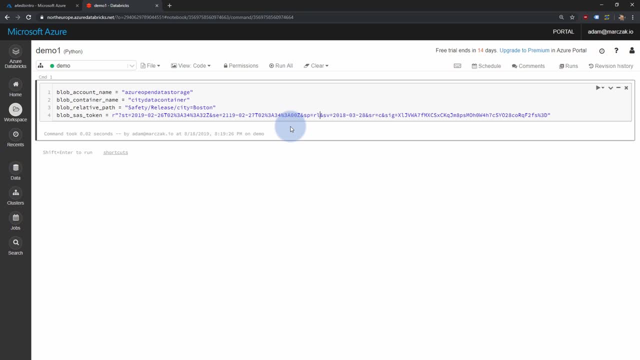 You can actually combine multiple blocks into a single notebook. To create a new block, you go here, insert new cell And paste new script. Oh sorry, That's the same script, So I'm going to copy the next one. This one is nothing to worry about. 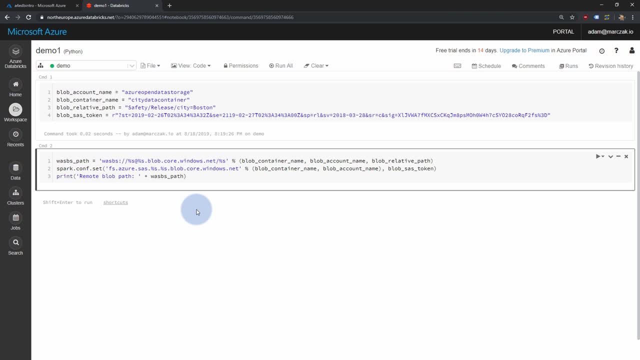 I would say this is the configuration that really needs to happen. Anyway, this is just for your information. This is the path to the blob storage. This is a very well not very user-friendly in terms of how to combine this, But documentation very nicely specifies how this should look like. 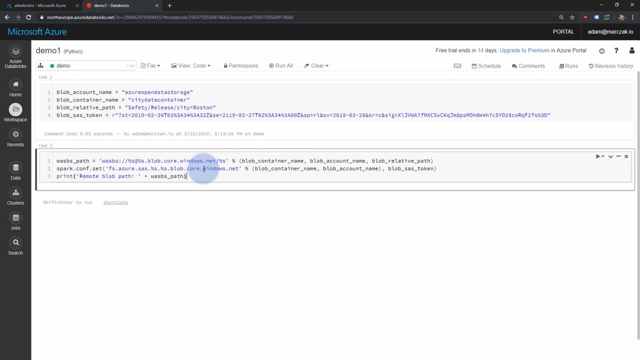 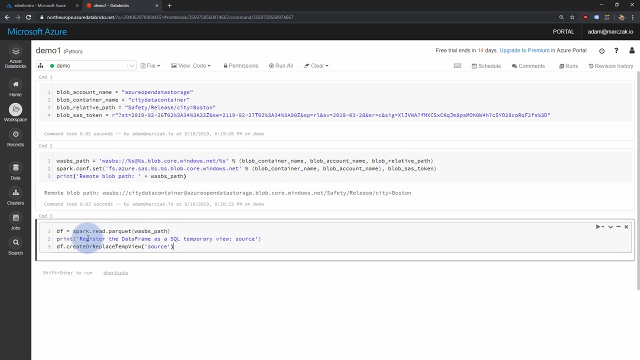 so usually just grab this from example and replace some values. so we just need to run this. so that means our remote blog path is blog protocol: ct data container: azure, open data storage and safety release city, boston, right, so let's grab data from this container. i'm gonna grab the next script and it says spark. 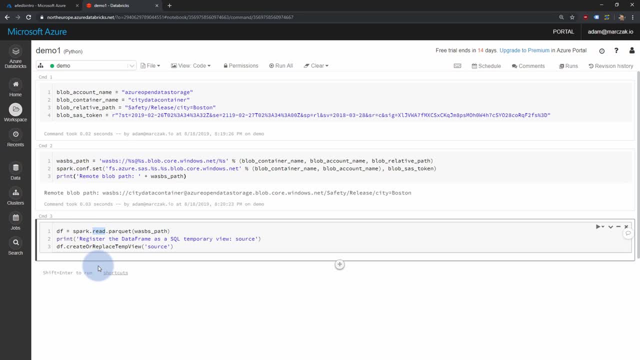 read. so basically we're telling spark to read the data. next we're gonna say parquet- this is the format of the data. it's just like csv or json file- there's also parquet files- and do it from the path from the previous step, then print some information and create the view. a view are used if you want to. 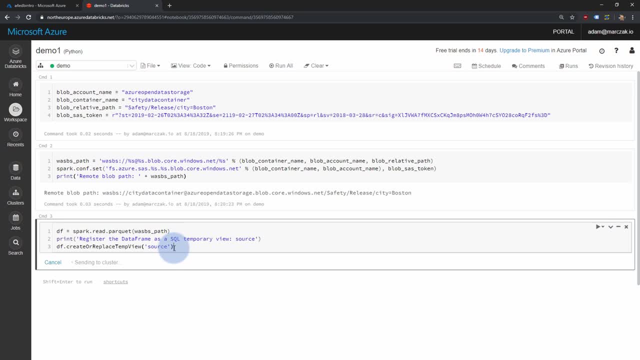 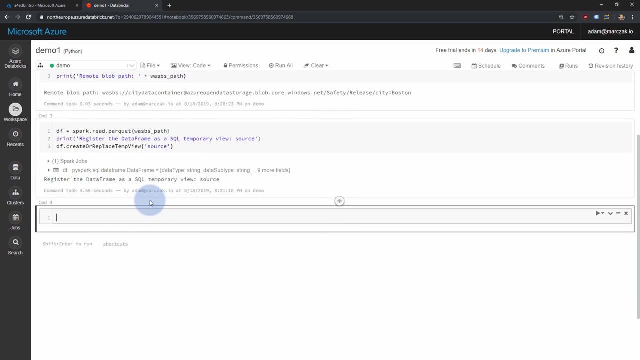 use sql, so let's hit control, enter and run this in about five to seven seconds. we should get it date combined. it was actually a bit faster force- under four seconds. so if this work right now, we can go to the next block and maybe display something about this data. what i'm gonna do is maybe i'm gonna 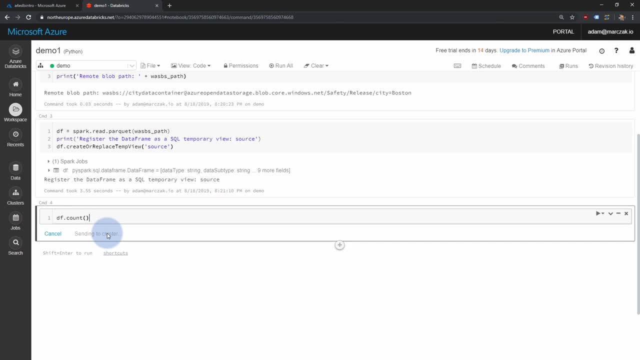 count those rows of that data, so i'm gonna hit ctrl, enter and run the job. so we have 127 000 rows of data that we read, that we can already work on, and, since we created a view called source, we can also do one of those powerful things that i was talking about, which is switching. 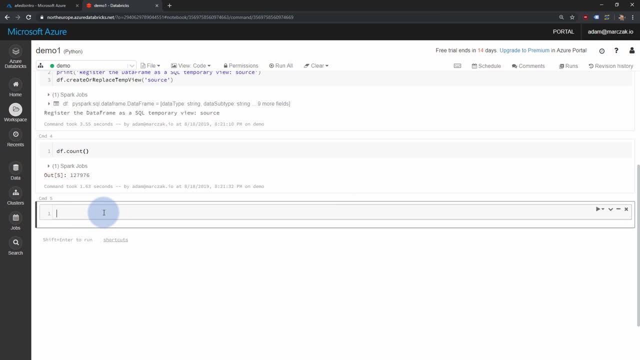 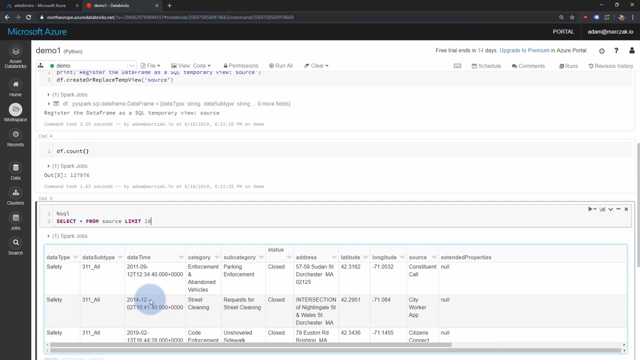 language. to switch language, you just type percentage sql and when you do that, you can start typing your sql comments like this: so select star, which grabs all the row from the view called source, and only grab the first 10 rows. hit ctrl, enter and see the results. it's really cool that we are able to connect to external blob storage. 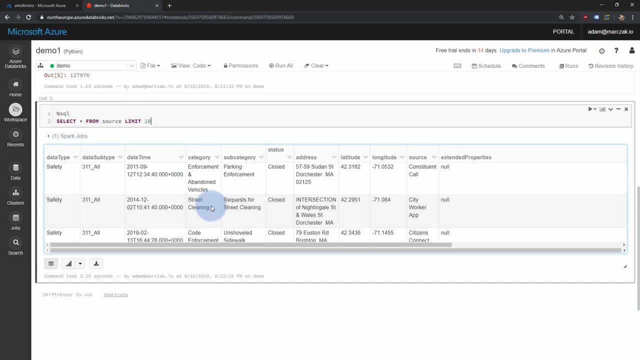 use sql to query the data and display it on the screen. but what's more is that if you're the analyst and you're doing this data analysis, you can grab your data here using download csv file and maybe pass it along to someone, or maybe hit this button and visualize it using bar chart or 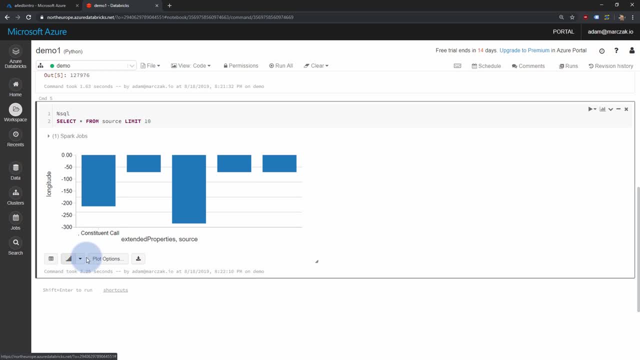 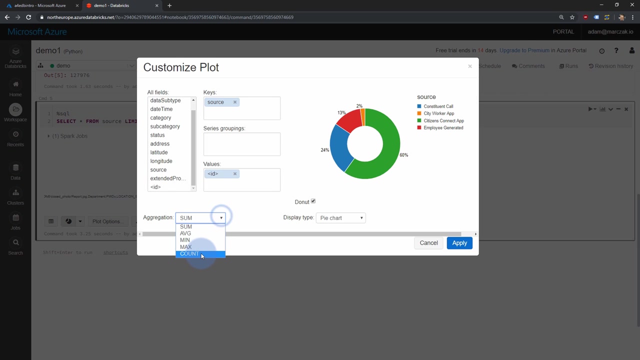 maybe look for a pdf file channel that you want to use as well. so let's go ahead and run that be a pie chart. of course, as pie chart you have additional options, just like in excel in pivot tables. you can use those here and change the values, maybe change the aggregate to count. 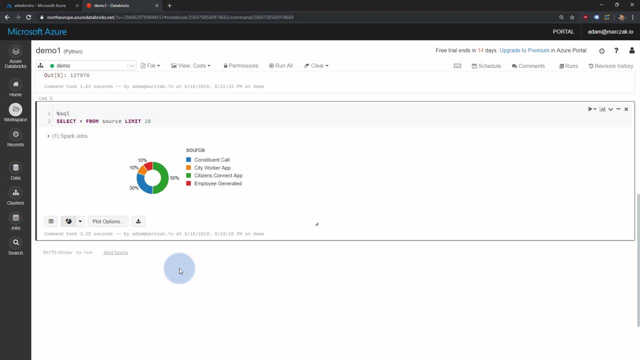 and hit apply and this is our chart. it's pretty cool, isn't it? so that was the demo for the python let's. i don't feel like this demo really shows what we did, because we not only use external storage, but we use very quick comments. we got some results, so i do really want to do more tangible. 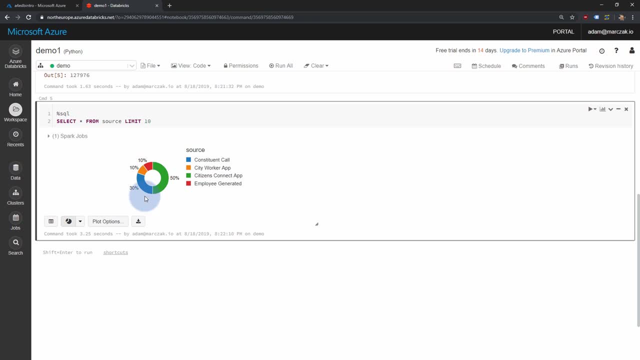 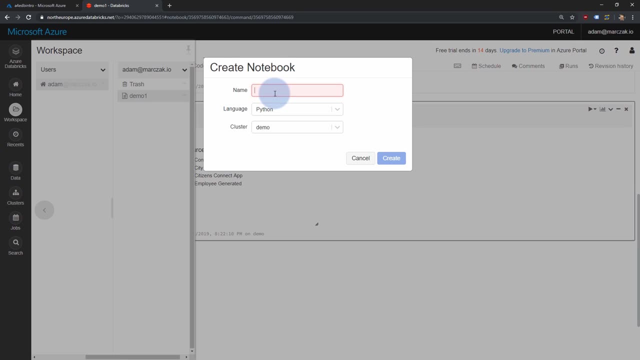 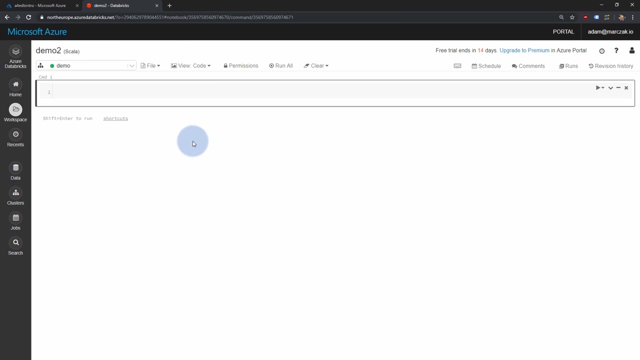 more hands-on experience with scripting. so we're gonna create one more script in scala. so let's go to workspace, right click, create new notebook, call it demo 2, and this one's gonna be in scala. so what we're gonna do here is we're gonna first upload our 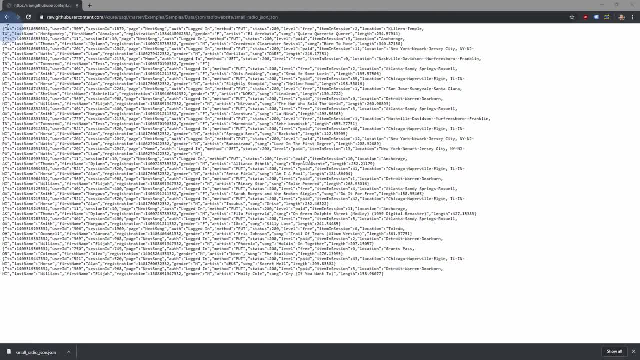 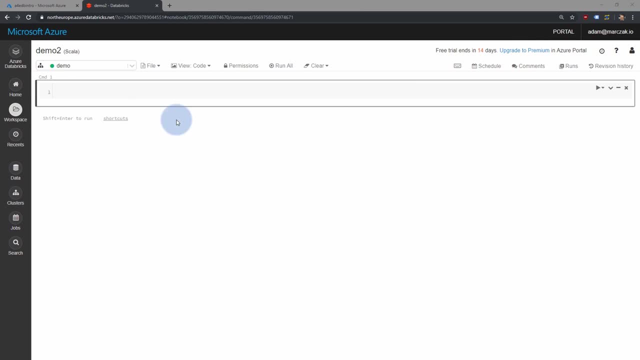 own data. so what i'm gonna do is i'm gonna upload those rows of data. there's 25 rows of data saved here as a json file. this is small radio json information. so i already download this, downloaded this file, so what i need to do right now is go back to azure, go to my resource group, go to the storage account. 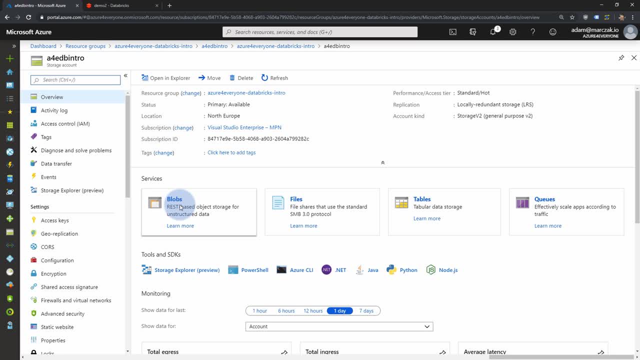 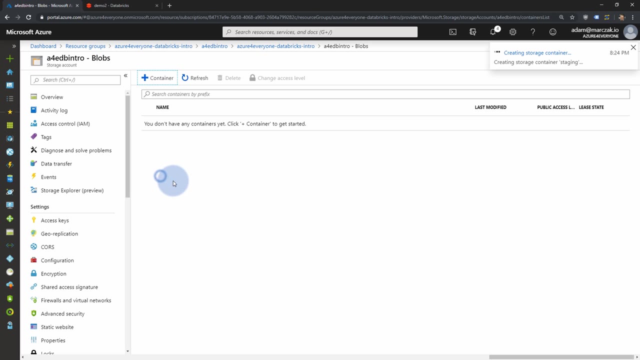 that i created, and this is the reason we created it: because i want to have this place where i can put my own data, transform it and put it back. so i'm going to go to blog service, create new container, i'm going to call it staging, i'm gonna leave it as private and i'm gonna go to staging and upload my file called small radio json. 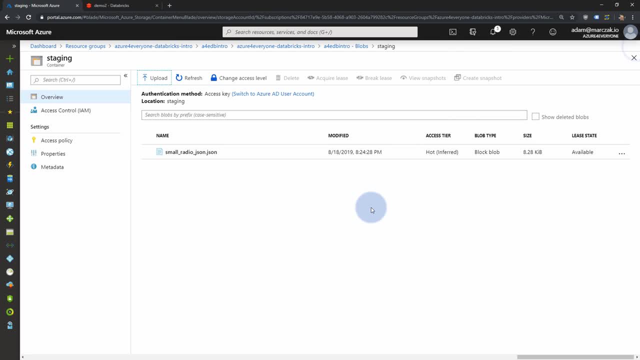 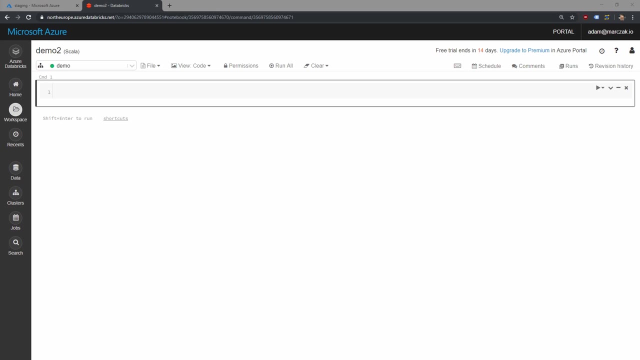 and upload it. so it uploaded successfully. right now we have on our container small radio json file. that's it what we need to do in this session. right now. we'll go ahead and should be able to kind of to do in terms of azure: let's go back to scripting. so this time we're writing code in scala, so i 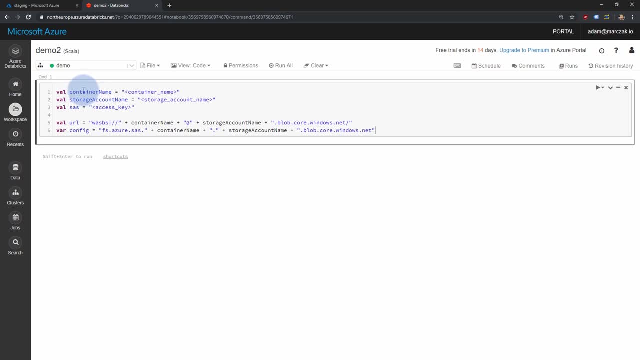 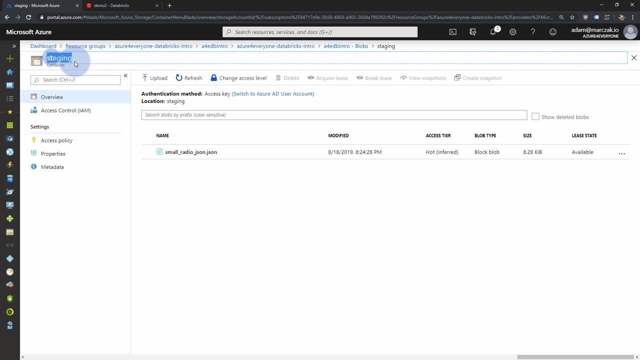 prepared some of the code already, so first of all, for this code to work, we need a container name, storage account name and sas token- the same token that we were given by microsoft, so we're gonna generate that in a second. first of all, we need a container name. our container name is called: 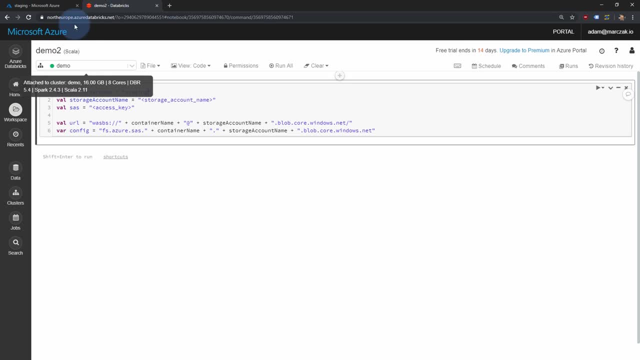 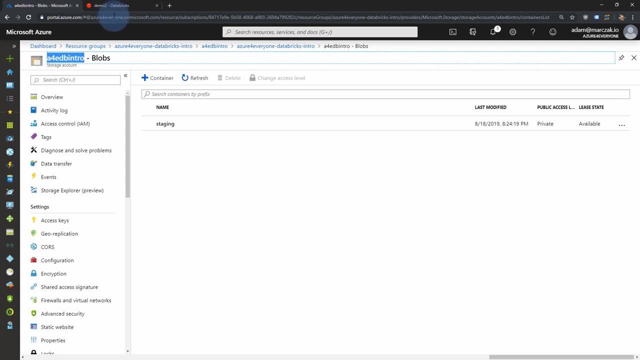 staging, so let's copy paste that and put it here. we need a storage account name, so let's go back and grab our storage account name and we need sas token. to get sas token, you go to blob service, go to shared access signature blade and select the service that you need to access to. i only need. 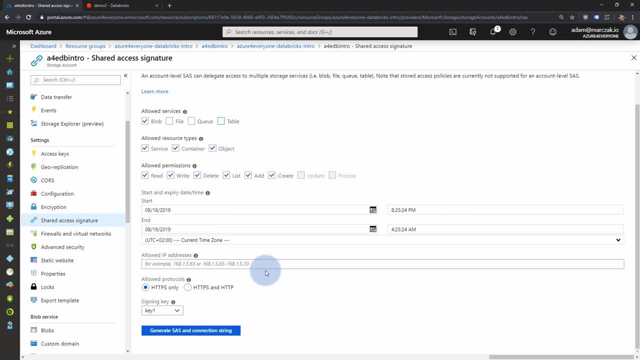 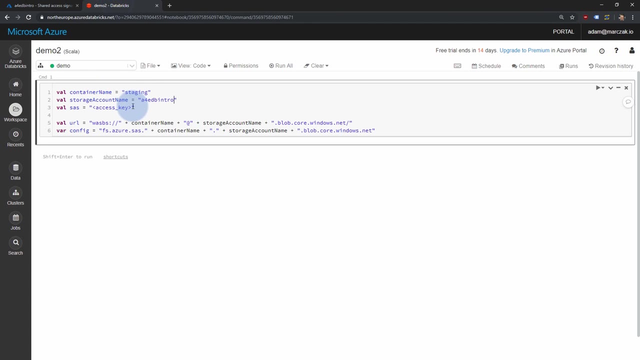 access for blobs. i'm going to leave it as blob and i'm going to leave everything else default. this means the storage that i'm giving access to has only access until tomorrow 4 am in the morning. so i'm gonna generate the sas, i'm gonna copy it to clipboard and i'm gonna paste it here. this is very. 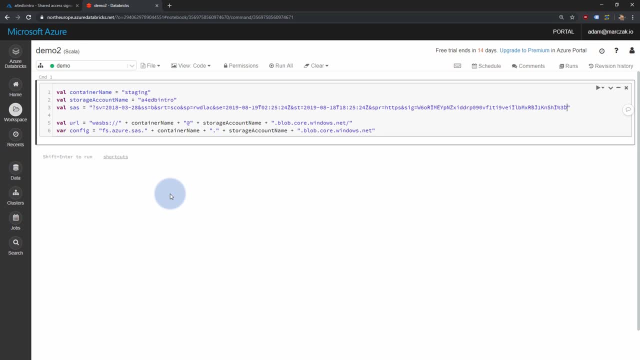 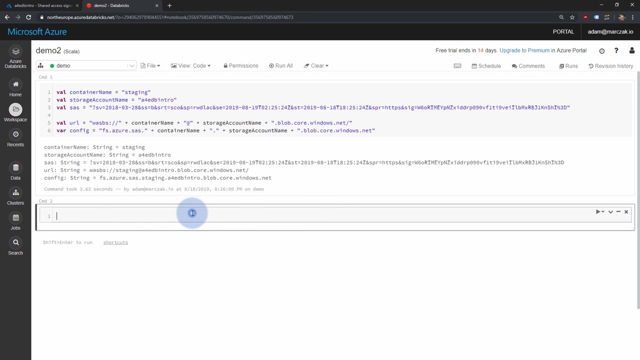 important that in this case this is very short-lived token, so if i would run this script tomorrow it would fail. so remember about that. i'm gonna hit control, enter, we're just gonna initialize those variables. i'm gonna hit plus and i'm gonna add new line. and this is very important. what i'm gonna do right now. 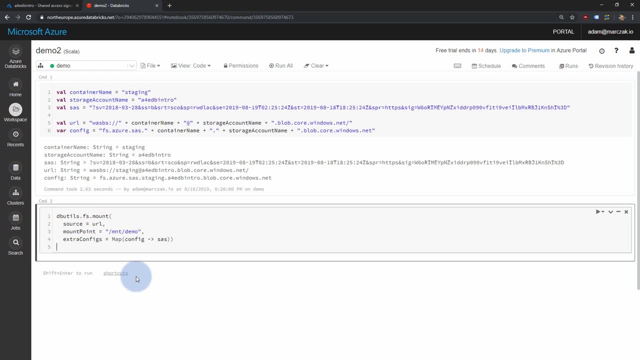 i'm using databricks utilities to mount a storage. so, just like you map your normal drive on your computer or windows or linux, we are doing the same thing here, except instead of mutting a drive, we're mapping a blob storage. this is a very, very cool feature, because using just normal windows shell- i sorry, linux shell- 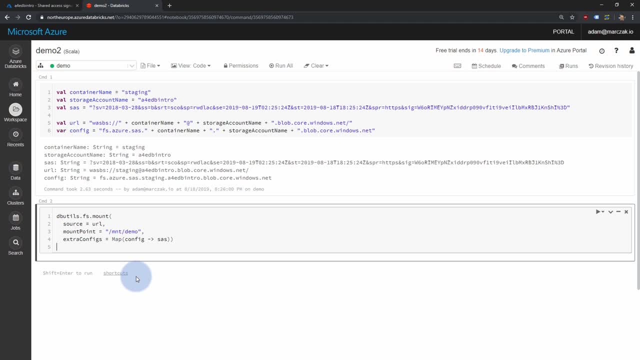 commands: 12 inefficiently empowered commands: дел Ал Tre клиàn VP development can copy theaha data to this mount and it will land on the blob storage. so I'm gonna hit ctrl enter this. sorry, let's rename it differently. let's call it staging. I'm 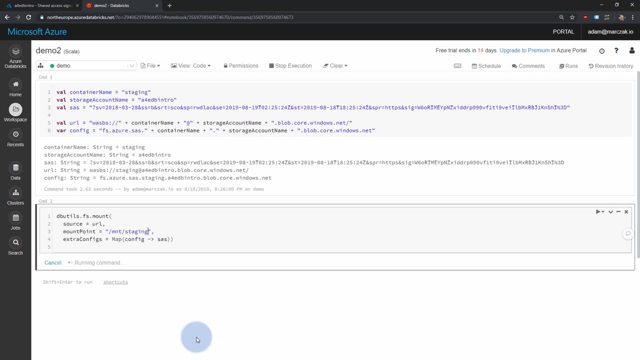 gonna hit ctrl enter, though. the reason it fell? because I already had a demo mount month before, because I was testing this scenario, so let's call it: staging this command takes about 23- 24 seconds to mount it, and from this point onwards, we will be able to use this mounting point to load our data after almost 22. 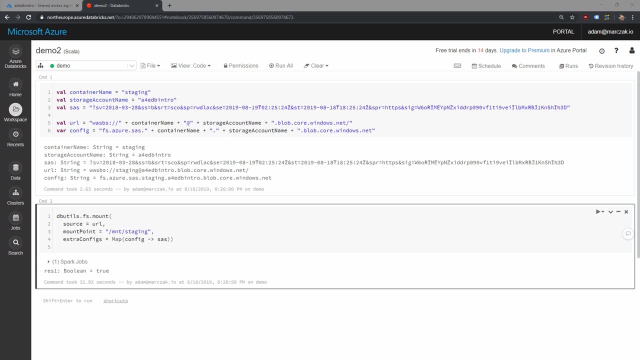 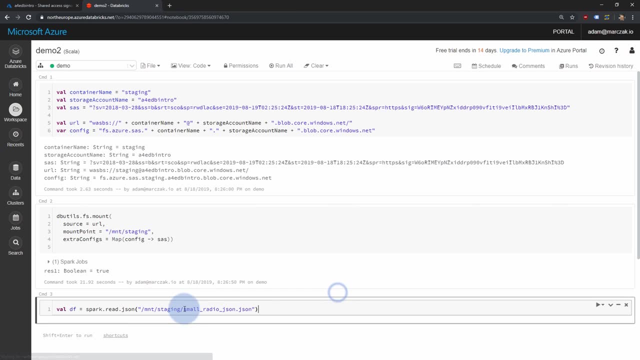 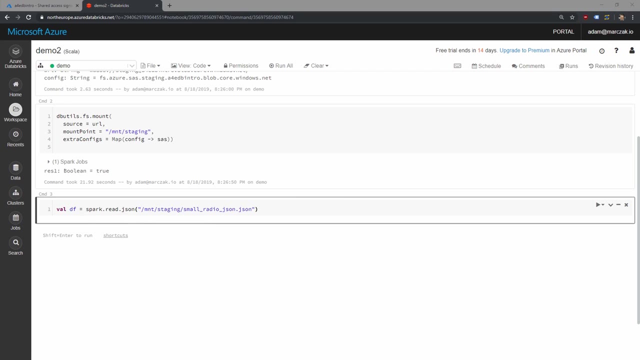 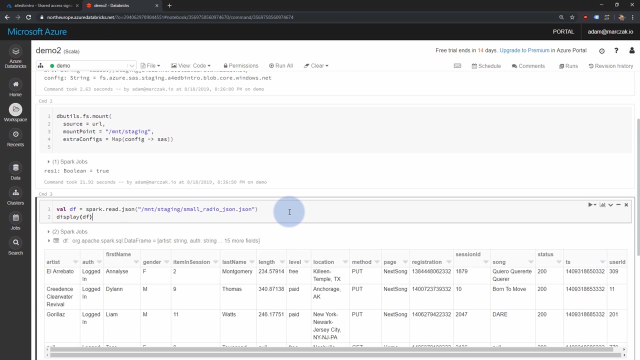 seconds. our staging is ready, so let's grab another line of code. I'm gonna grab a line of code that will allow me to read from a mount slash staging small radio Jason, and what I'm gonna do is I'm gonna display this data and hit ctrl enter. so 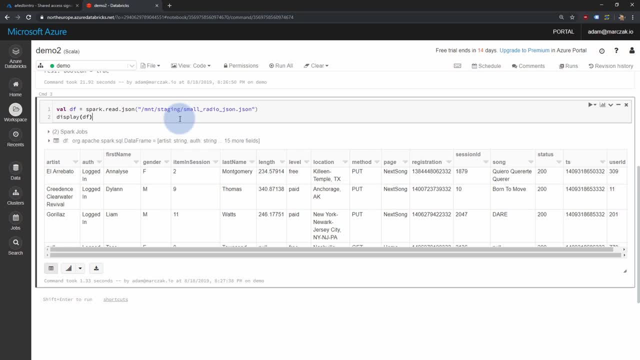 as you see, it was really fast. but what is cool here is we used it like it would be normal file on our Drive, except it was on a blob storage and yet we were able to connect, load that data and display it. it's very, very cool to be. 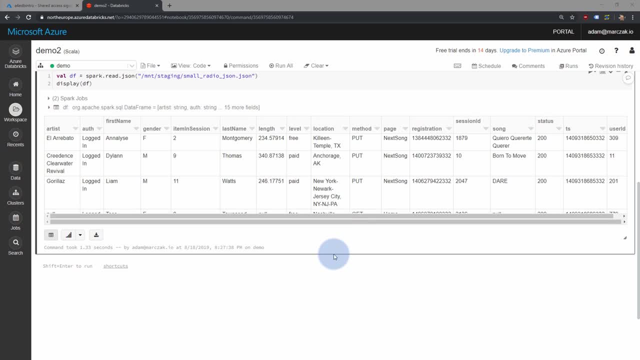 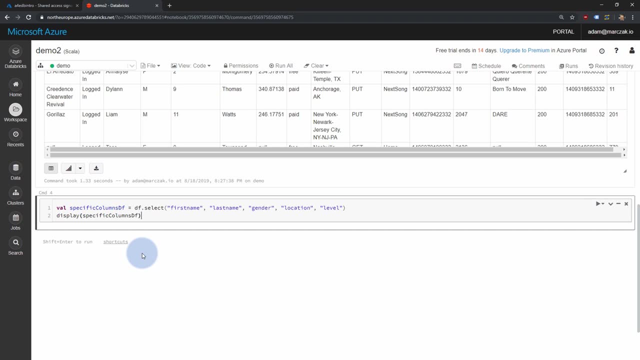 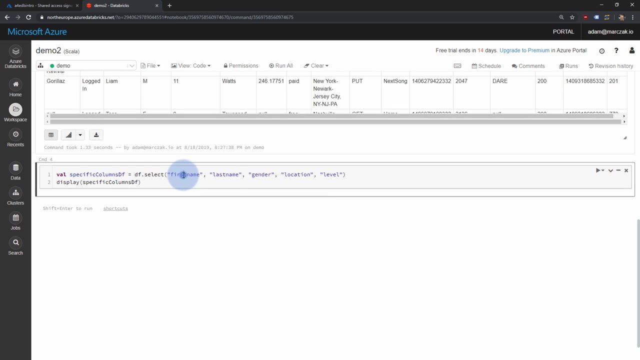 honest. next, what we're gonna do is gonna create another block and paste it in, and then we're gonna add that class factor to our layer below it as well, and here we're gonna use a select statement. this is a similar to selecting this cue, well, where we're rubbing our data frame consisting of our data and selecting. 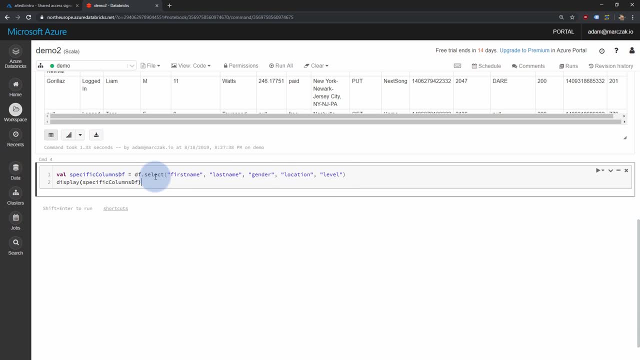 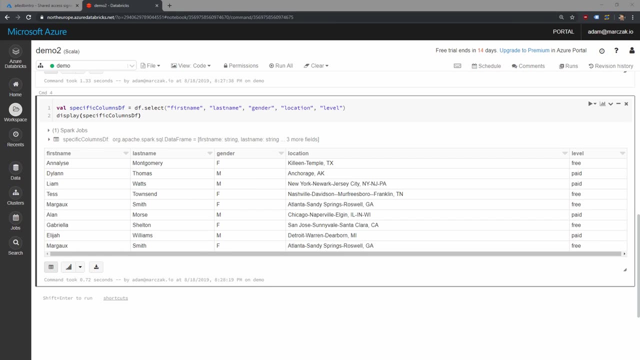 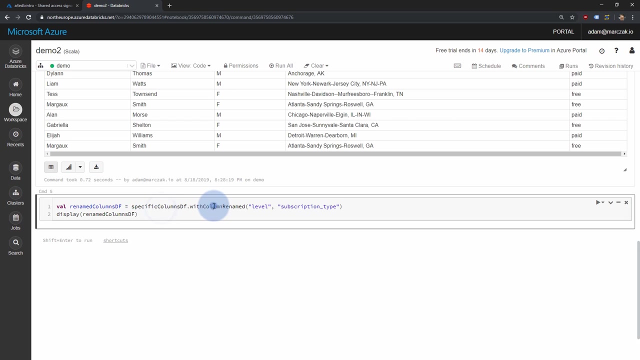 only few columns- first name, last name, gender, location and level- and displaying that data frame to see the results. hit ctrl enter. everything seems fine. that was the first transformation that we did using data bricks, so let's do the second one. a saved previous step specified specific columns, data frame and from this result i'm grabbing and. 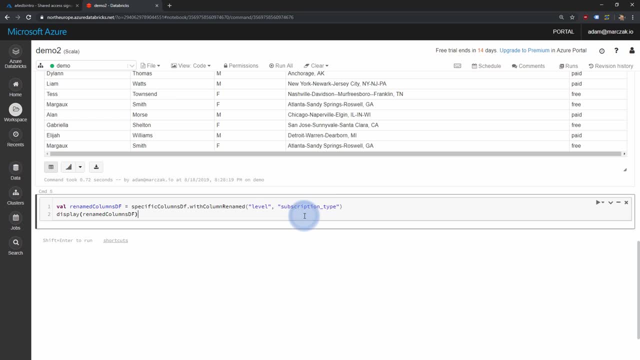 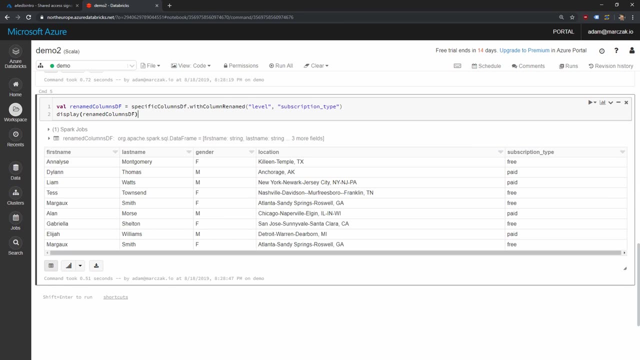 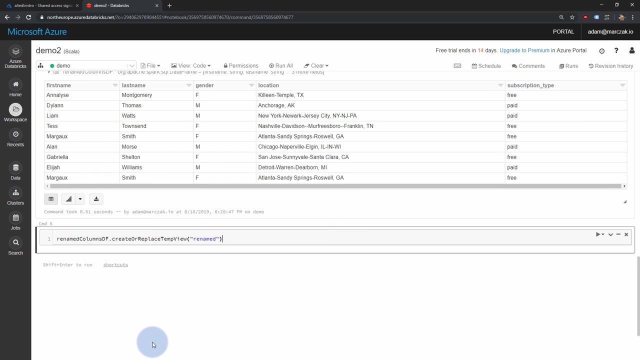 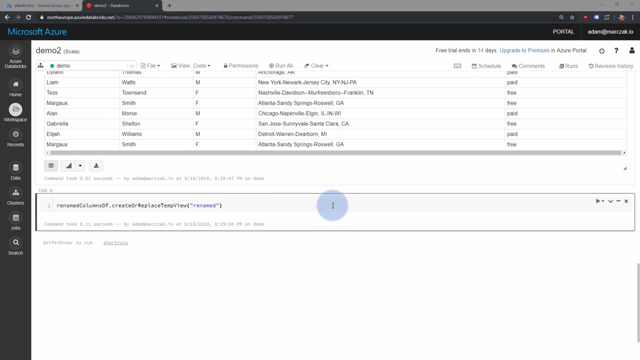 renaming one of the columns called level to subscription type. let's hit control enter and again see the results. the column was renamed. what else you can do here is the same as previously. maybe let's create a view called renamed control enter and the view was created. so how about we do some simple aggregations, maybe count how many subscription types are there? 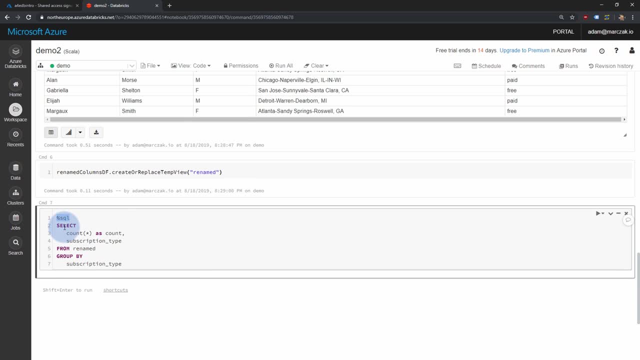 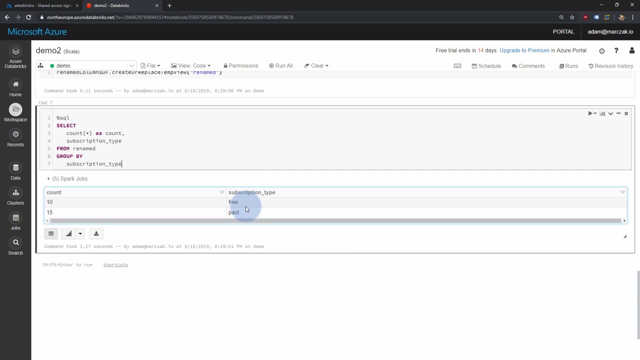 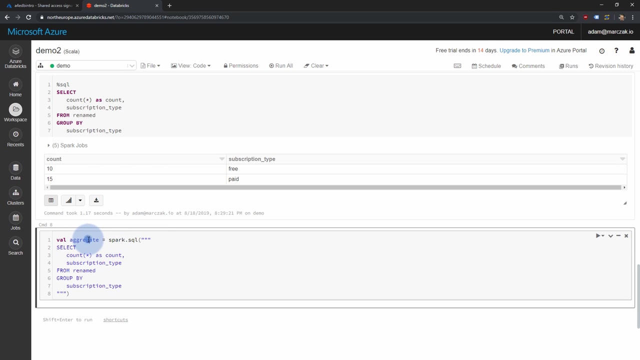 so i'm gonna type percentage sql and select count by subscription, type, hit control enter and we got 10 free subscription and 15 paid ones. and if you want to save this as a result in in some data frame later on, you just encapsulate this select statement into spark sql and assign it to aggregate variable hit. 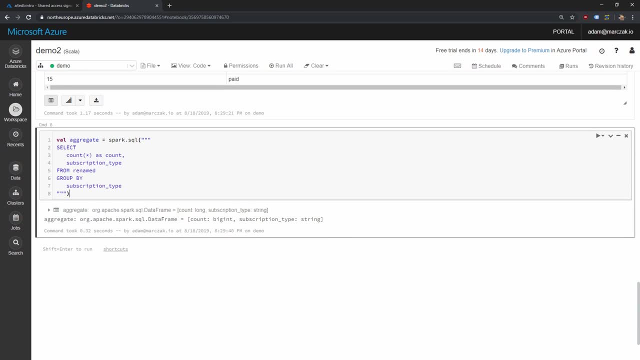 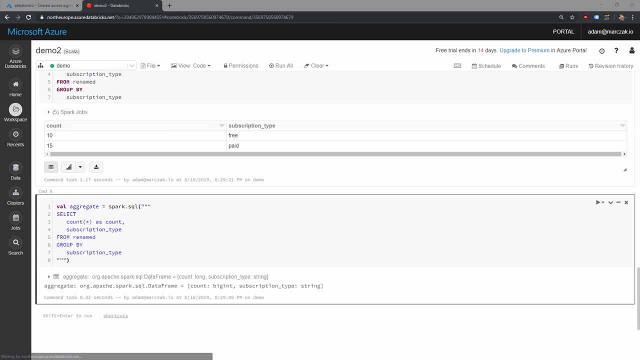 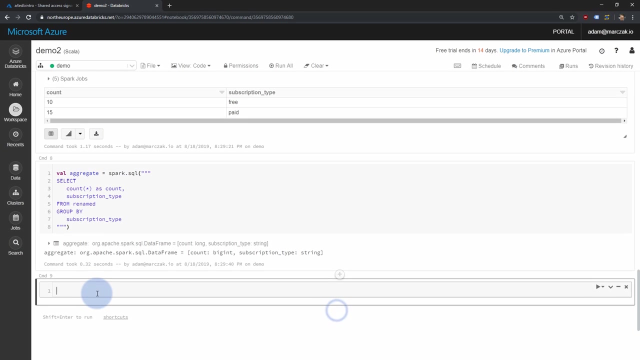 control, enter. and now in aggregate variable we have a, that aggregation that we created a second ago. so since we have that, we can already go further and maybe save that on a blob storage. let's grab one more line and grab aggregate. so the result from the previous step. 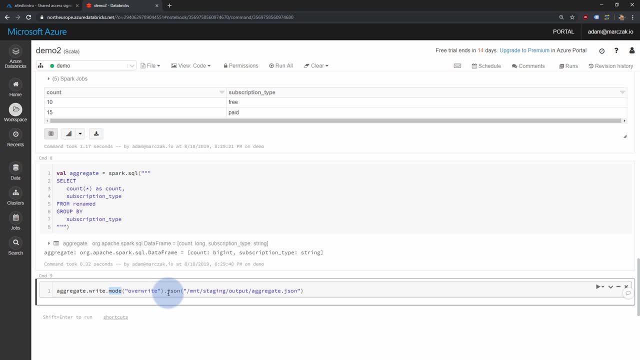 right mode overwrite. so if there are any results on the blog search existing already, overwrite them. write it as a json file. so this is the specification of the format. it's pretty much as easiest changing this to csv and we're gonna have a csv file, so let's hit control enter. and it finished. so if it did finished, we can control, enter it over here. and we have this clause now. let's say, this is the chicks liver text file, so if it changed here, if it changed to json file, it is finished. so if it changed but it's over here, we're going to have- we're doing this- one more timeament master in and would capsizing because it was something that we can do. but if we do that and we were going to use that to power over a subpar calculation for this 거, so let's grab, add subpar property. 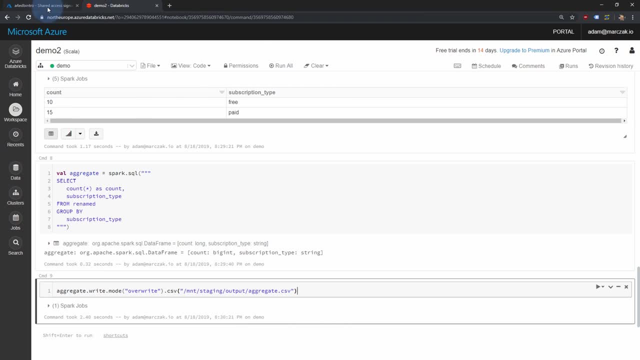 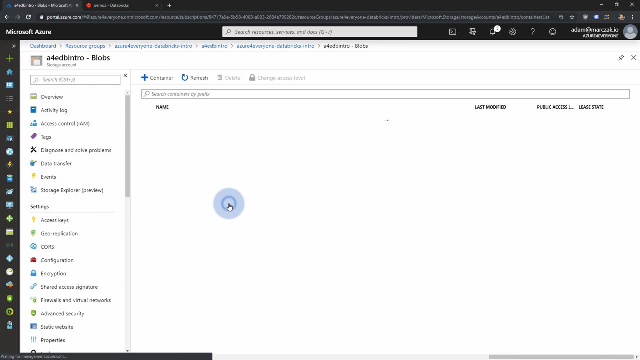 over want again take our го to knowledge. more questions, you… finish, and we didn't mess anything up. we go back to our blob storage. we go to the overview tab, go to the blob service, staging, open output- aggregate csv. we have a file that is empty. 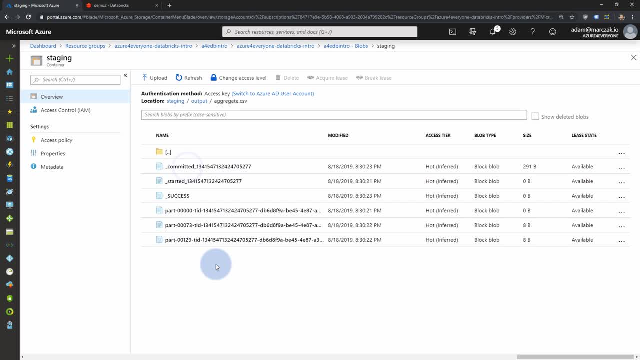 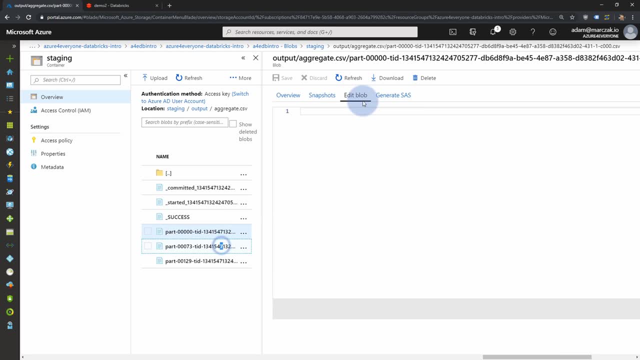 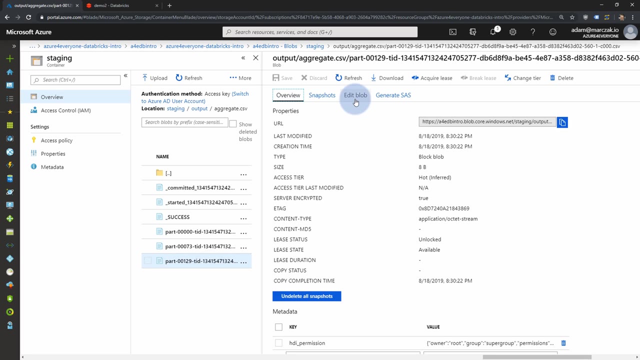 zero bytes, because this is just a metadata file and within the aggregate, we have some information here. but this is a splitted csv file. actually, sorry, this one. see, this is a csv file: 10 free ones and 15 paid ones. why is it split? because this is how spark. 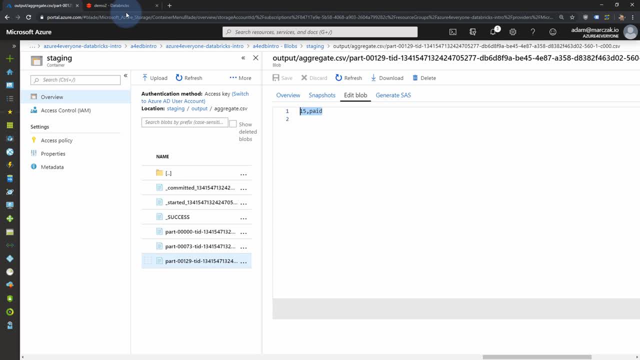 works. it's split: splitting data into partitions for more effective processing. of course, you can control that. if you want to have singular file, you can always combine this data using simple commands. but i just wanted to leave this as brief ones. what is cool is that data bricks and spark itself. 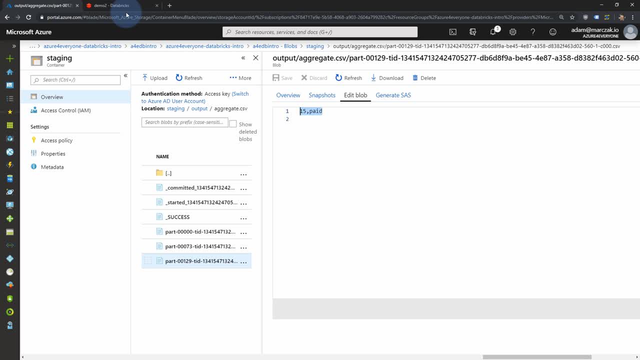 knows how to use those files and how to combine them in a singular data frame. the other files that you have here is success, which is the status of the processing. you have the started file, which says when the processing started, you have committed file. this is the file that says how many files did you create during this processing, says you see it. 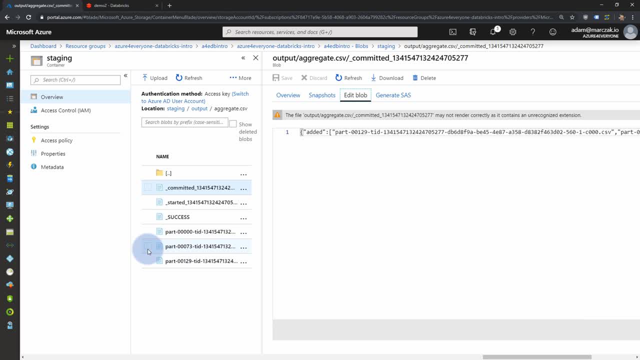 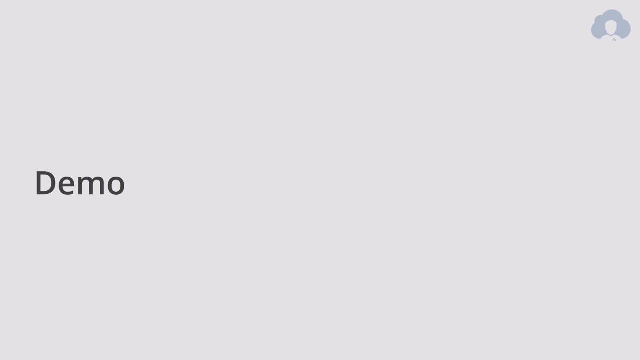 says we created two, so it's pointing to this- and this file. so this is how spark knows which files to pick during and that was processed and how to process this further. so if we go back to our presentation and talk about very last thing that we, just to summarize: 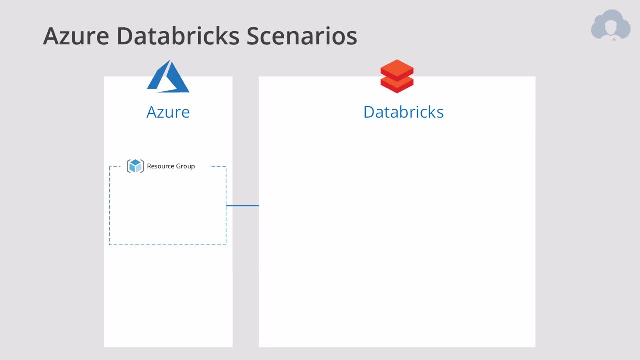 the information that we learned here. first of all, you have azure in azure, in the resource group you have databricks workspace. this is the resource that combines features about the service, but only very limited features, because in reality, you have the separate service in the portal called azure.